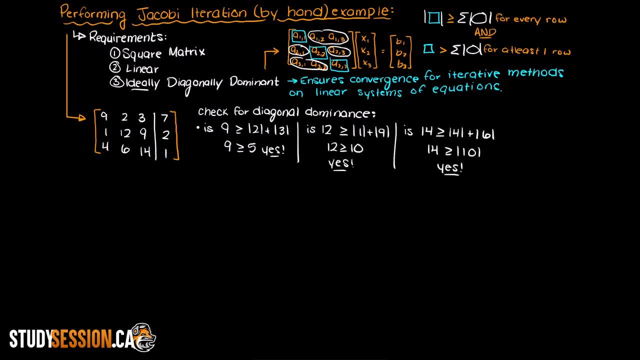 row. So, as you can see here, it is clear that our matrix is diagonally dominant. Therefore, no matter what we assume for our initial x vector, our answer will always converge. So let's begin solving this matrix using Jacobi iteration. 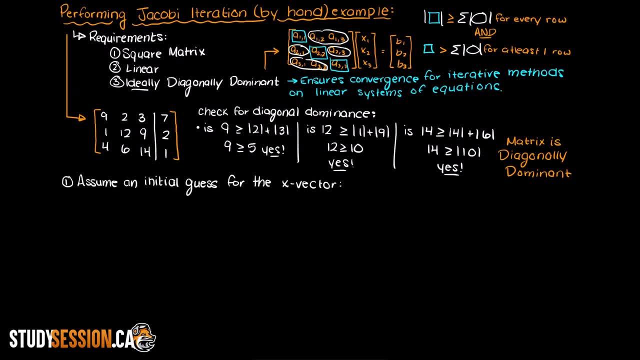 So, firstly, we need to make some assumptions about our x vector values Commonly. unless more information is given to you, a good starting point is just a zero matrix. So that means that all of our x values we initially assumed are going to equal zero. 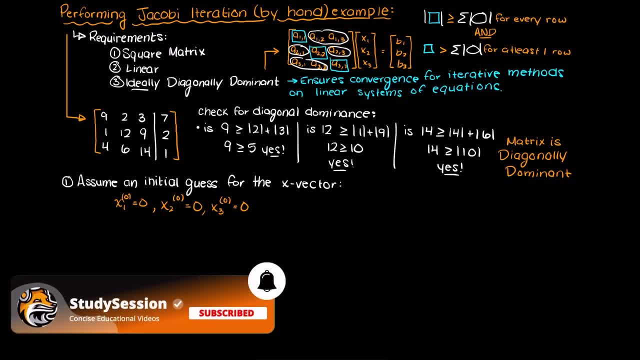 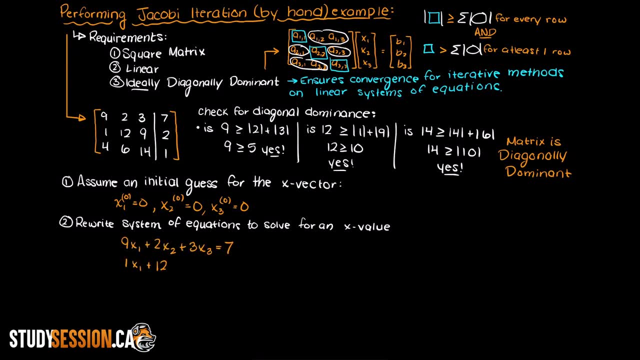 These values will then aid us to get our next iteration of x values. Now step 2, we must rewrite our independent equations in terms of one x value. So the easiest way to understand this, if you are a bit confused, is to actually write out the equations like so and then solve for the 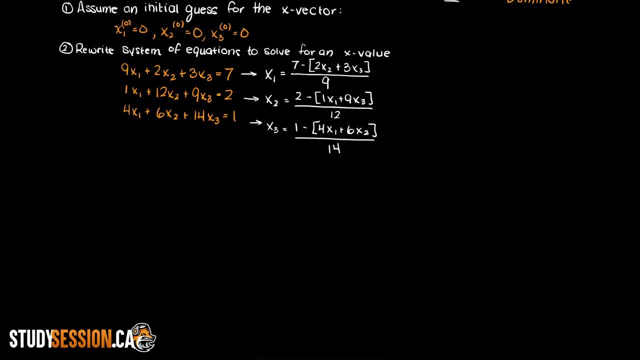 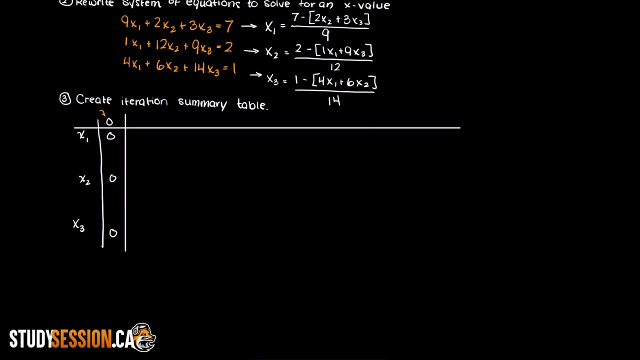 x value. Now, as you can see here, every one of our independent equations is now solving for one of our unknown x terms. Now let's create a simple table where we can keep track of all of our x values at every iteration. Now we are ready to begin solving for iteration 1.. Just as a side note, 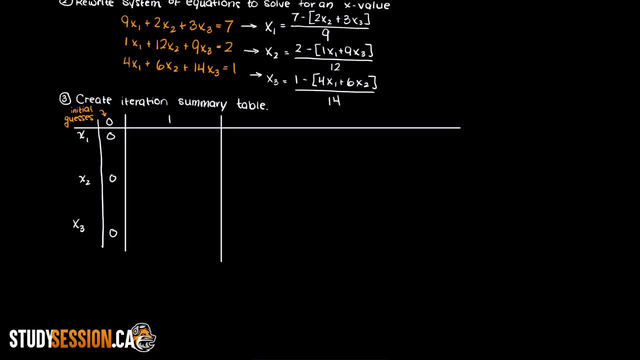 iteration 0 is really up to you. If you are using MATLAB, for example, you would typically call your initial guess iteration 1, as MATLAB does not use zero indexing, That is, all counting begins at 1. Whereas in, say, Python, all counting begins at zero. So if you were developing a program in 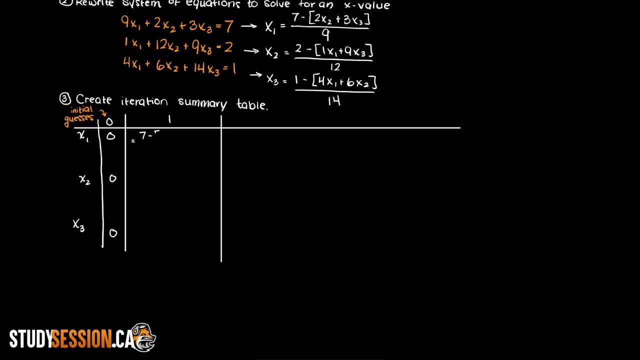 Python, it would make sense that your initial guess is labeled zero. So let's plug in our assumed x values into these equations like so, And we will receive a list of x values that are going to be our guesses in our next iteration. Now we continue this process until we reach a sufficient 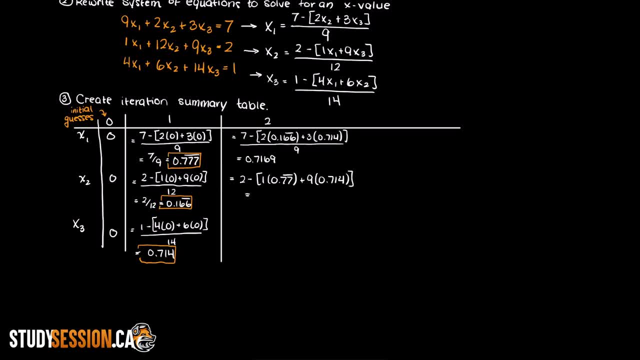 level of accuracy. This part is much easier in computer programs, as you can just tell the program to check every step how close your x values will get you to the right hand side of each of your equations. Just pause the video now and try to perform a couple Jacobi iterations on your own. 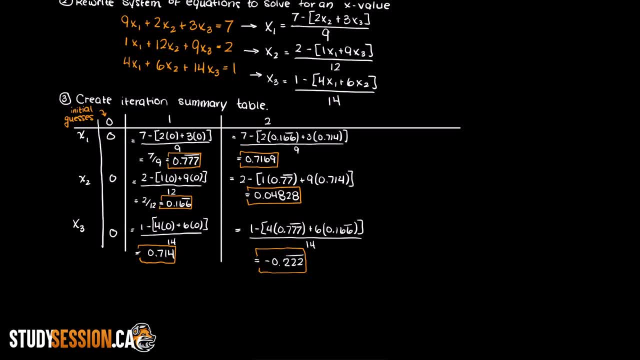 like we just did to make sure that you actually understand Alright. so, after 5 iterations, these are the x values that we arrive at. Although we could keep going at this point, I hope you have an understanding of how Jacobi iteration works. at this point, Let's validate that we are converging on an answer, though, Which you 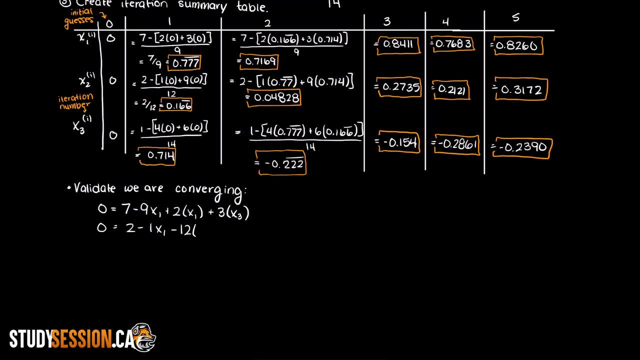 may have to do if you are doing this by hand, on a test, for example, Let's set all of our equations equal to zero and then plug in our x values at each iteration. I am just going to do this for equation 1, but the exact same process should be followed for the other two independent equations. 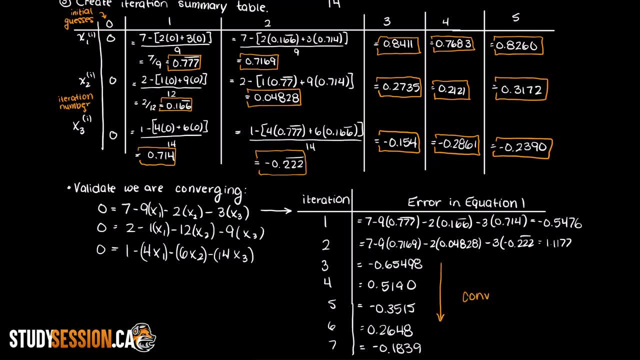 As you can see here, with every iteration we are getting closer to zero, which is exactly what we want. This proves that we are converging on a solution, And this makes sense, as we know that this should happen, since we validated earlier that our matrix is diagonally dominant. 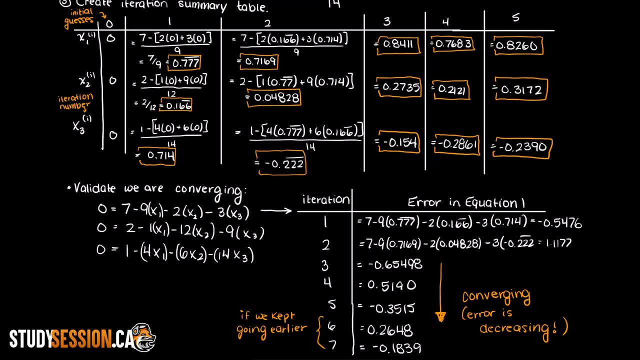 In the next few videos, I am going to show you how to perform Jacobi iteration in Microsoft Excel and using Python, as programming is a much easier and far less tedious way to solve iterative numerical methods. Thank you for checking out this video and I will see you in the next video. Bye. 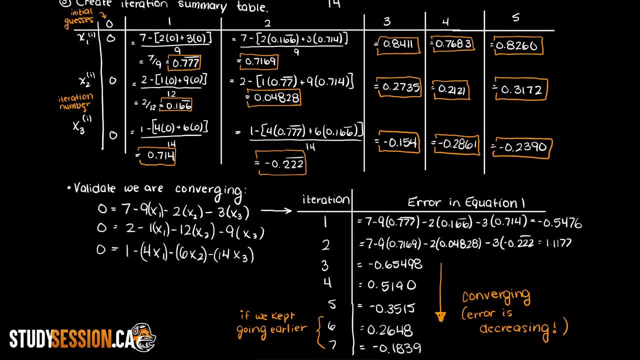 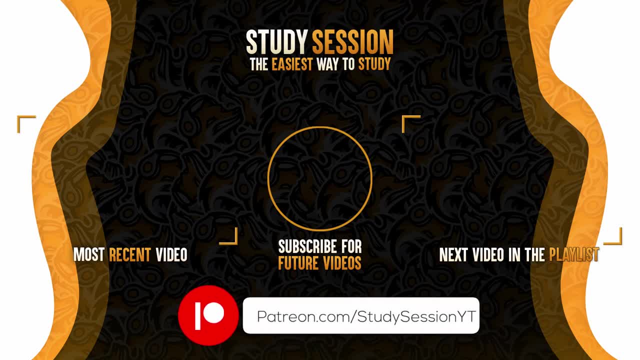 And I hope it helped your understanding of how we can solve systems of linear equations using the Jacobi iteration method. If you enjoyed, please like and subscribe to support the channel. However, if you have any comments, questions or concerns about the information I provided, 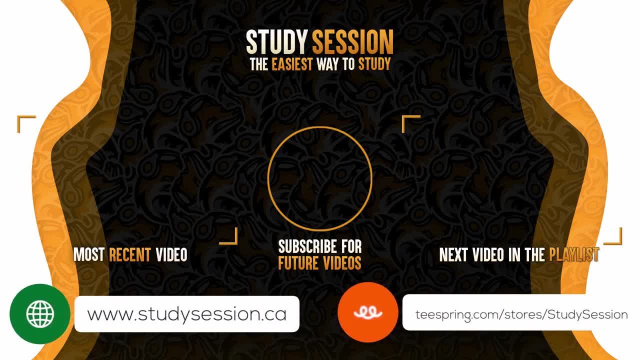 in this video. please leave a comment down below and I will do my best to address your concerns. 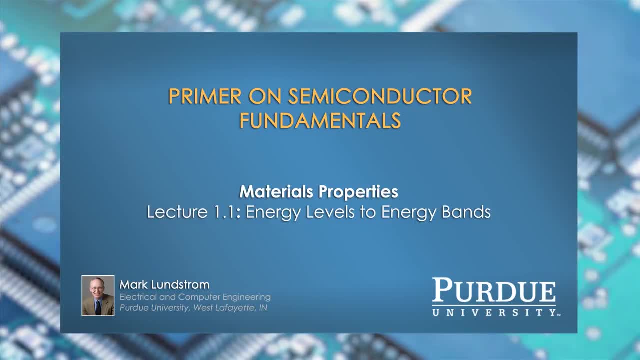 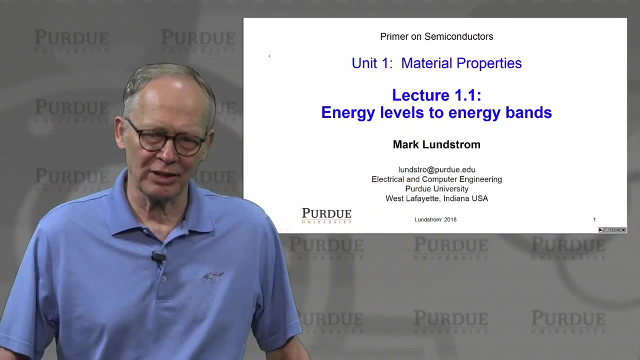 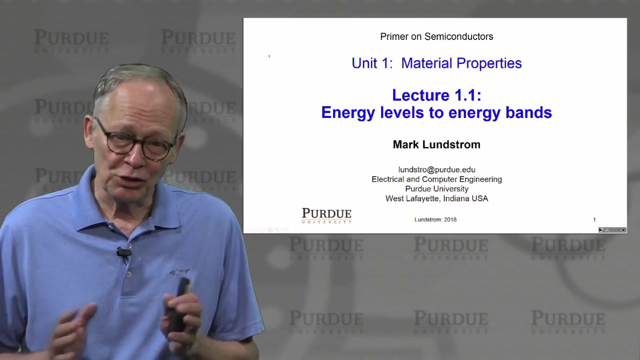 So welcome to this short course on semiconductor fundamentals. By the end of this course, you should have an understanding that will allow you to understand the operation of almost any type of semiconductor device. In Unit 1, we're going to dive right in and begin. 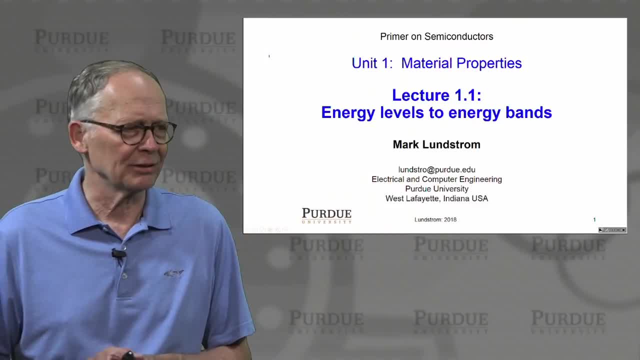 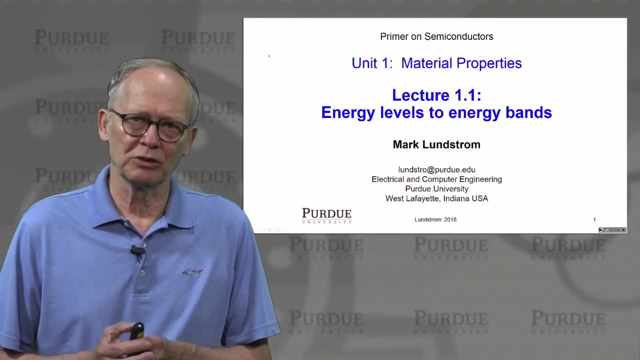 to talk about some basic materials properties of semiconductors, And I'll be relying on some of the knowledge you have from an undergraduate chemistry or physics course and we'll show how those concepts are extended and applied to real semiconducting materials.